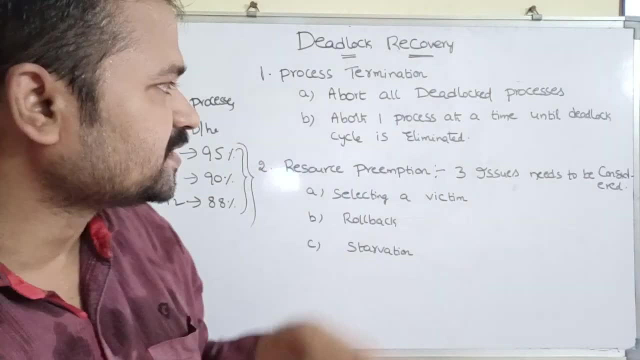 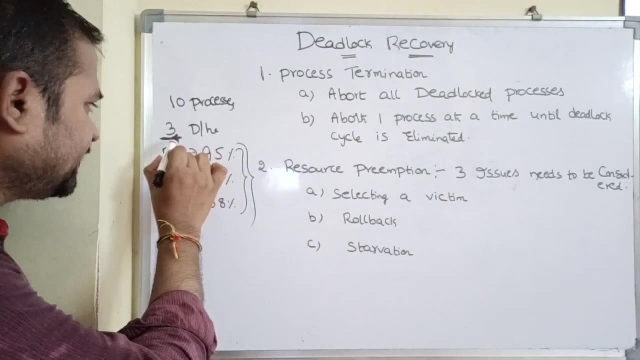 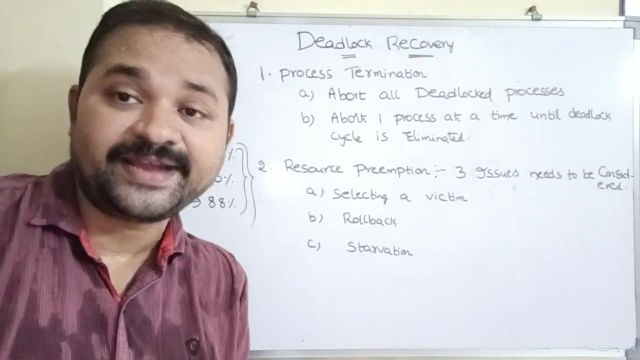 That is the first approach, And the second approach is about one process getting until the deadlock cycle is eliminated. So let us assume that here three processes are suffering with deadlock. So first kill the first process and apply deadlock detection algorithm in order to check whether the deadlock cycle is eliminated or not. 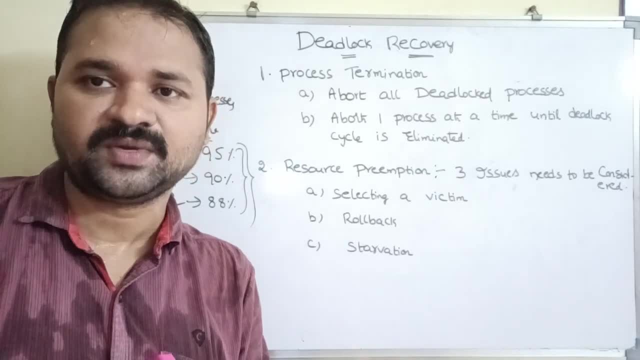 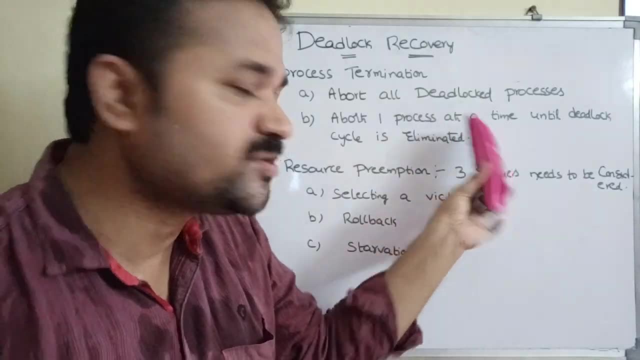 Suppose if the deadlock cycle is eliminated, then there is no problem. Suppose if still there is a cycle, then we have to kill the second process from the, the second process from the system And again we have to apply deadlock detection algorithm in order to know whether the deadlock cycle is. 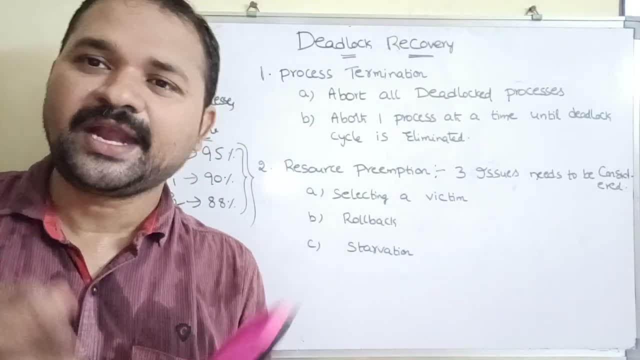 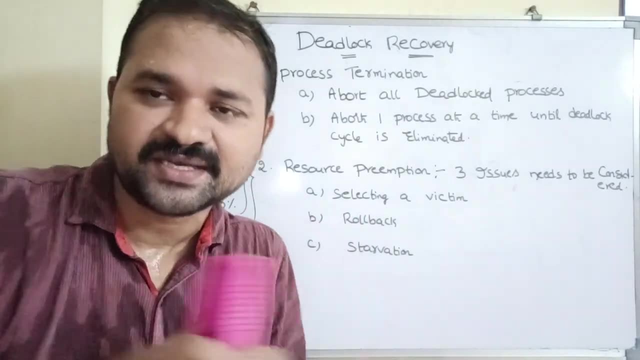 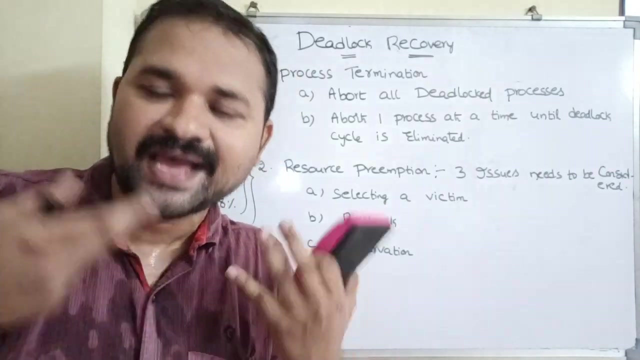 eliminated or not. Let us assume that there are 100 processes that areBlue which are suffering with deadlock. then, after killing the first process, apply deadlock detection algorithm to check whether cycle is eliminated or not. again, we have to kill one more process and we need to check whether cycle is. 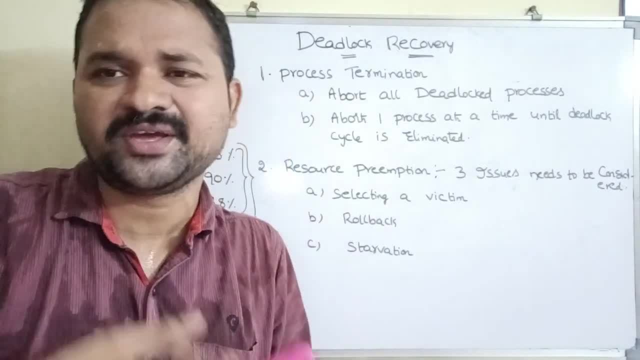 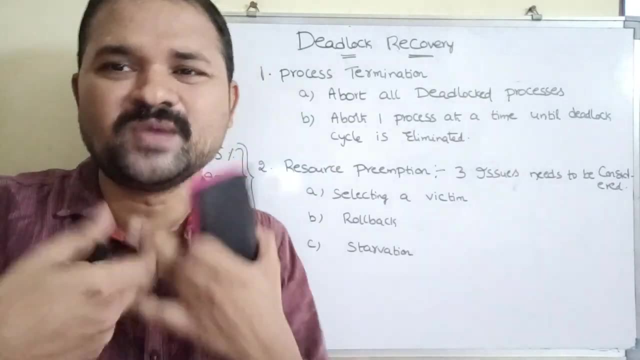 eliminated or not. so here there is a too much of overhead on the computer. why? because we are applying deadlock detection algorithm every time after killing the process, so there is a too much of burden on the computer because of too many deadlock detection algorithms needs to be applied on the 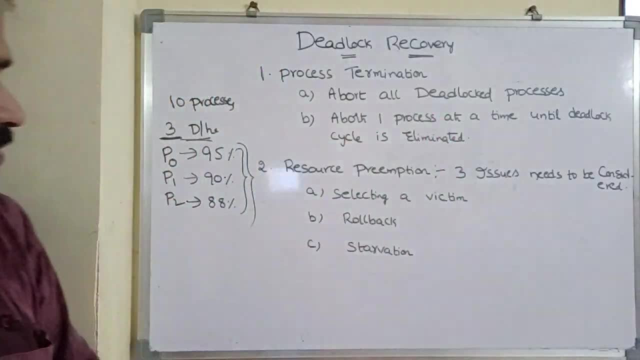 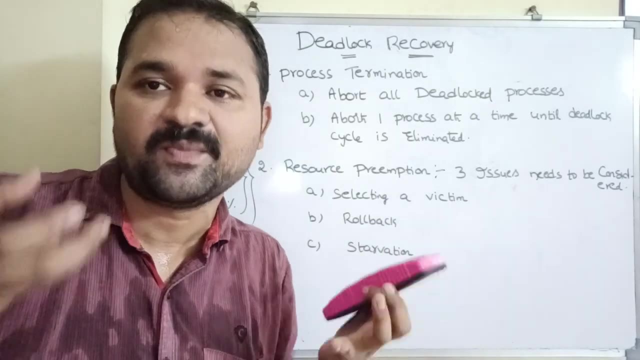 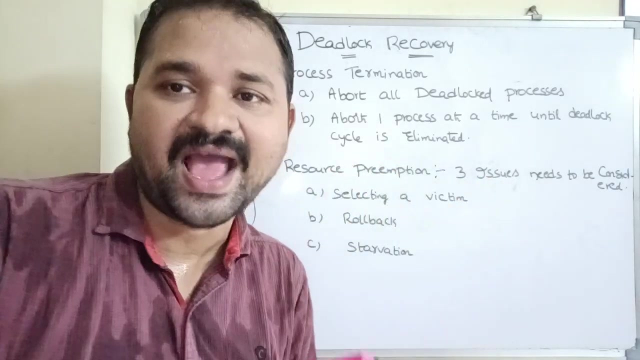 deadlock cycle. ok, so this is the disadvantage of this approach. so which process we have to about here? we have several processes, so which process we have to about now? that needs to be considered also. so we have to kill the process with low priority if you have high priority processes and low priority. 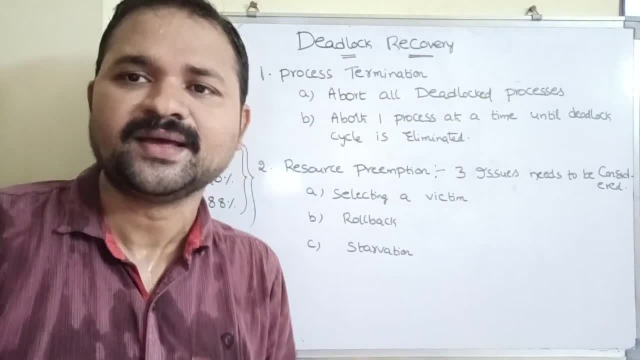 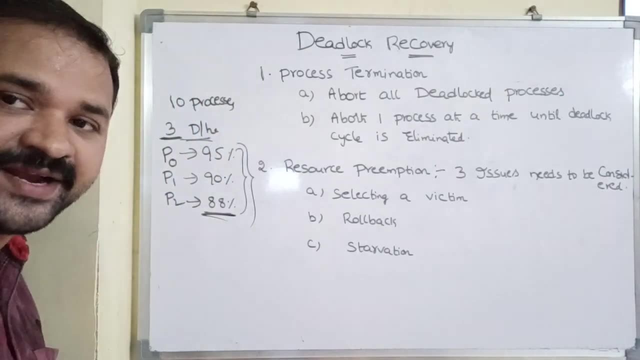 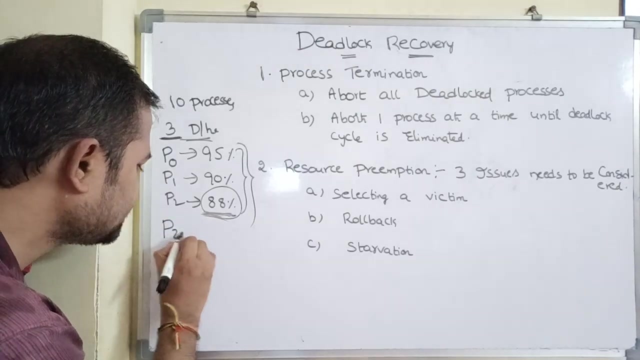 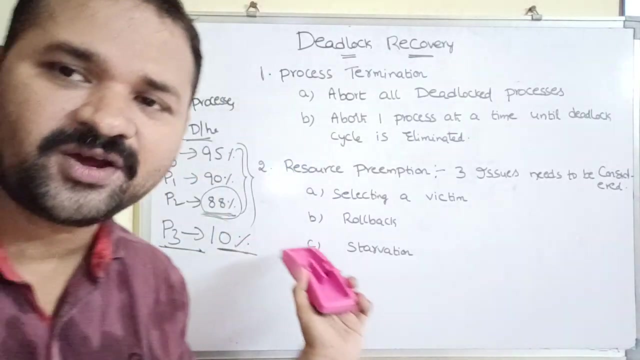 processes, then it is better to kill the process with low priority than high priority and kill the process which which is executed for the less period of time, which is executed for the less percentage of time. let here we have one more process whose execution time is completed, only 10%. then it is better to kill p3 rather than killing peanut, p1, p2. 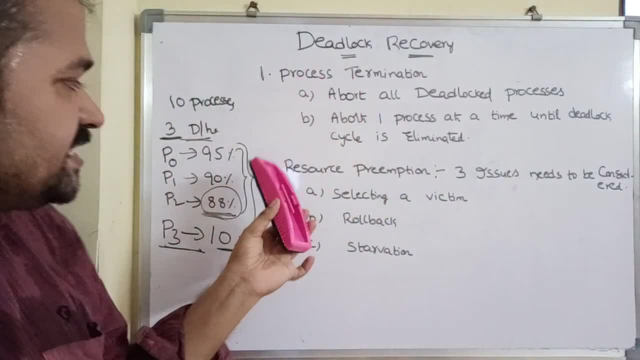 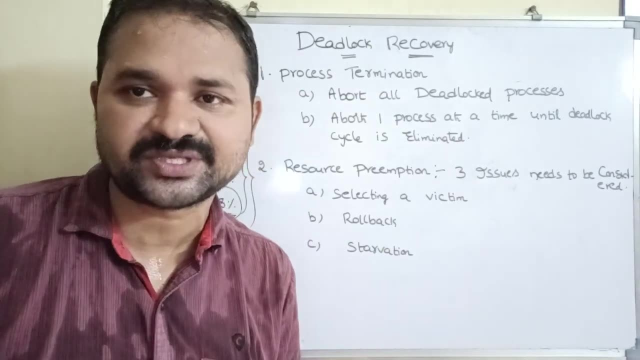 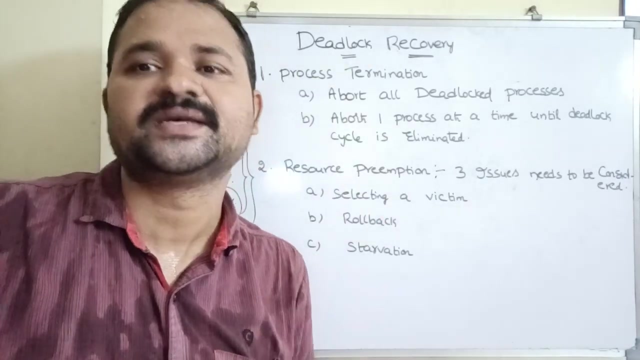 so we have to consider those issues. now let's see about the second approach. that is nothing but resource preemption. so preemption means releasing the resource. so here we have to release a resource from the process and we allocate the corresponding resource to the process which needs the corresponding resource.